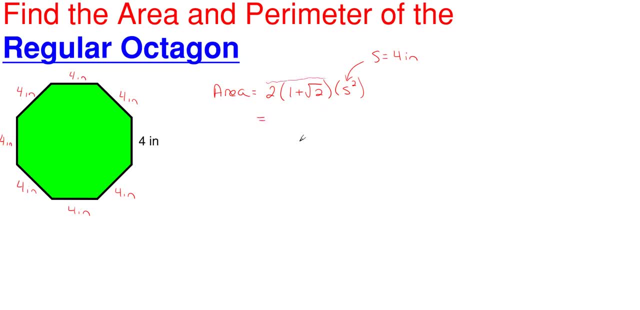 So my area, since this portion right here is constant, it will never change, based upon whatever your side is, Two times one plus the square root of two will always be 4.828.. And then the second part will just be times S, times S. So this: 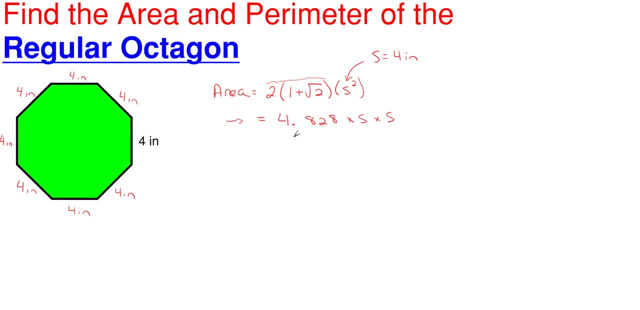 is the area equation that you will use. It will always be for a regular octagon: 4.828 times your side times your side. So, filling this in here, we will have 4.828 times four inches, times four inches, And this will give us a value of an area for. 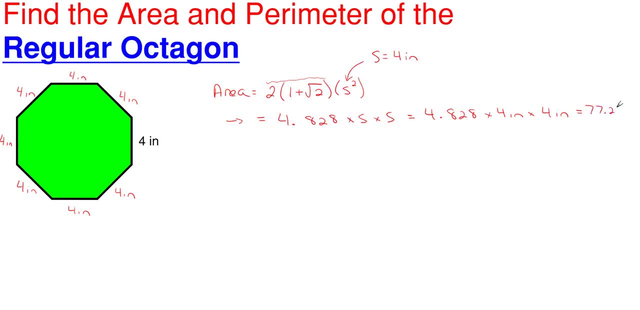 this regular octagon of 77.25 inches squared. So that's how much area we have in green inside this regular octagon. Keep in mind that your units have to be squared here. They have to be an inch squared because anytime you have a square root you have to have an inch squared. So 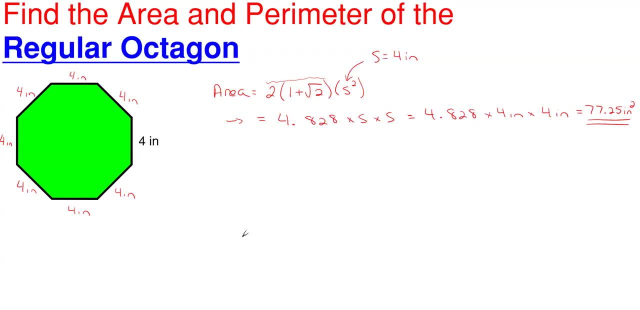 this is a unit that is being squared, that represents area. So let me just reiterate real quick that this 4.828, right here and here, will always be that value depending upon. it does not matter what your side is. Our side here was four inches, but if it was two centimeters it would. 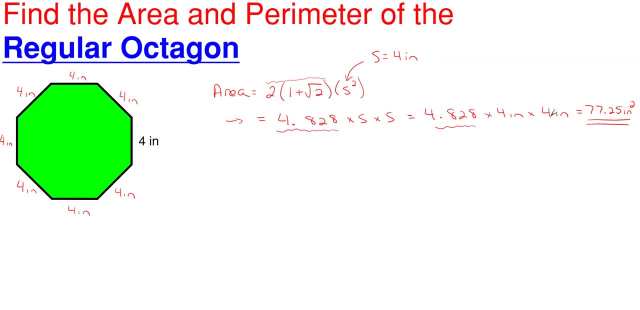 still be 4.828 times your side, times your side, whatever one of your sides is. So that was how you determine the area. Now, looking at the perimeter. well, the perimeter is just a fancy way of saying how much distance does it take to get all the way around this thing from. 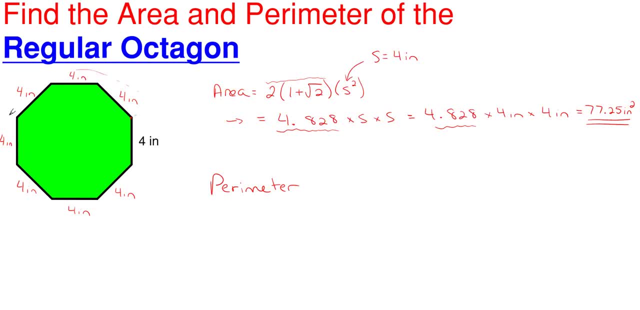 your starting point ending at the same point. So we're just going to work our way all the way around this, and how long and what kind of dimension does it take to get there? So all of our sides are four inches, So we are literally going to just add four inches together eight times. So we would 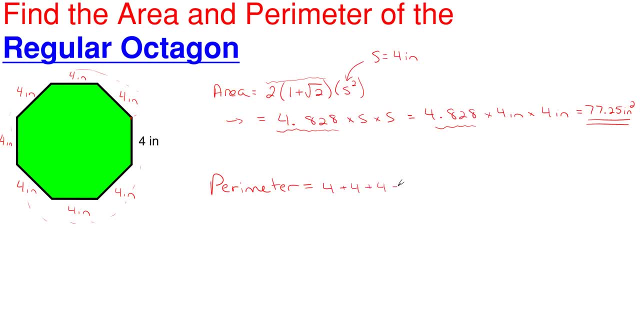 have four plus four plus four plus four. Let's see what's that. six plus four And there's our eighth four. So adding four together, eight times gives us 32 inches and a distance to get all the way around, our regular octagon.